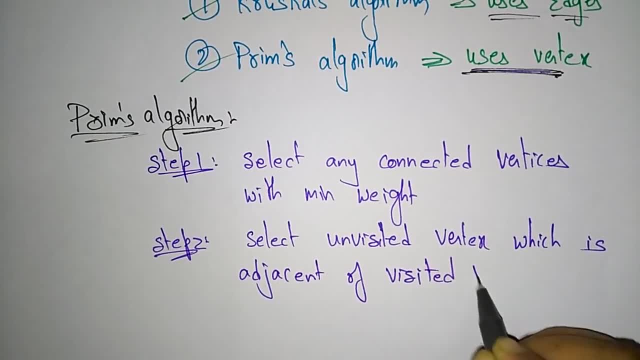 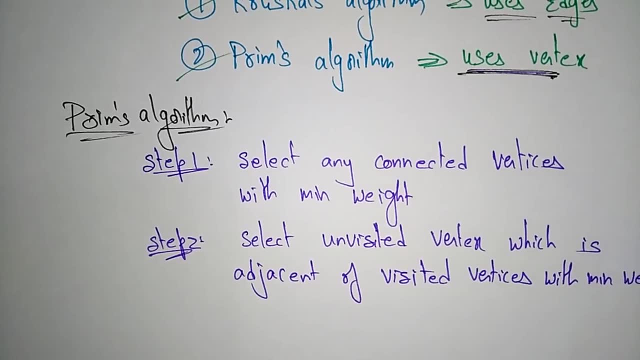 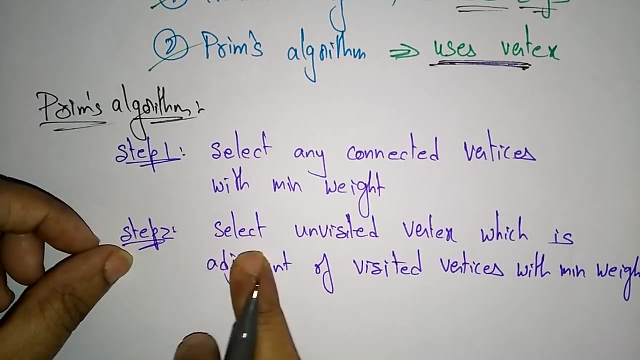 Adjacent of the visited vertices with minimum weight. So that is the rule, Because first we have to select any one of the vertices that is having the minimum weight in the edge And the next in the step 2, we have to select the unvisited vertex but which is adjacent to the visited vertex. So it should be like here or here, or here means which is adjacent. 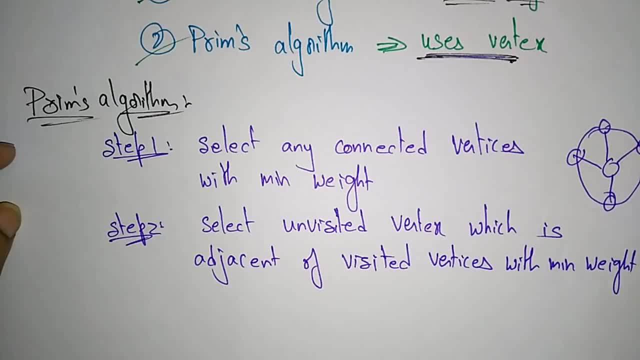 Adjacent, Adjacent to the unvisited vertex. Adjacent to the visited vertex? uh, visited vertex. so this is a visited vertex and we have to select the unvis unvisited vertex which is adjacent to the visited vertex, and that to that vertex should be with minimum weight. 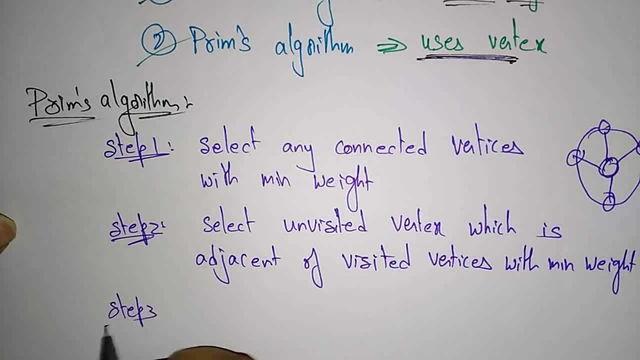 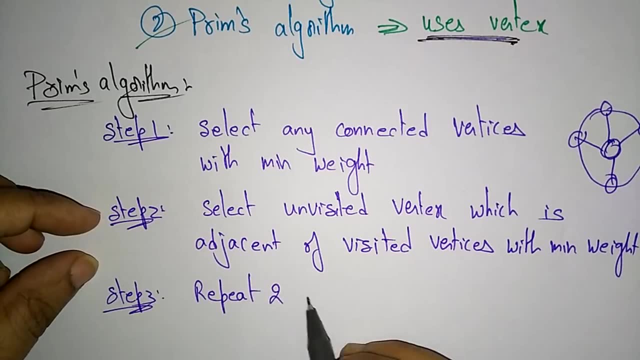 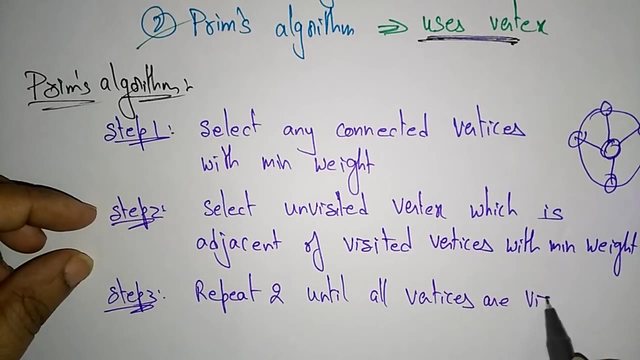 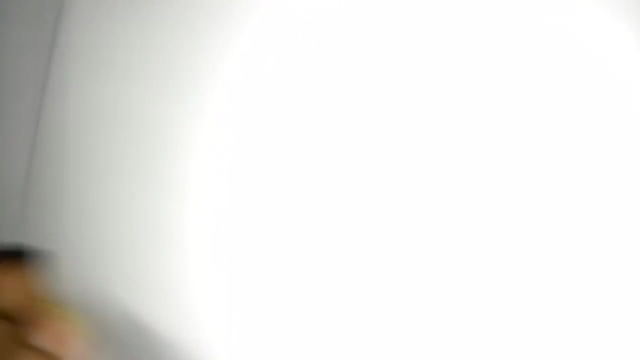 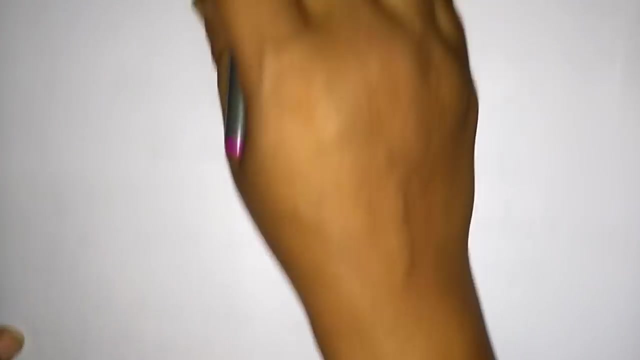 that should be minimum weight. and step three: we have to repeat this step two until you visit all the vertices. repeat step two until all vertices are visited. okay, now let us see one example by how this prints algorithm. well, so we will apply this algorithm on this example. let me take the example. 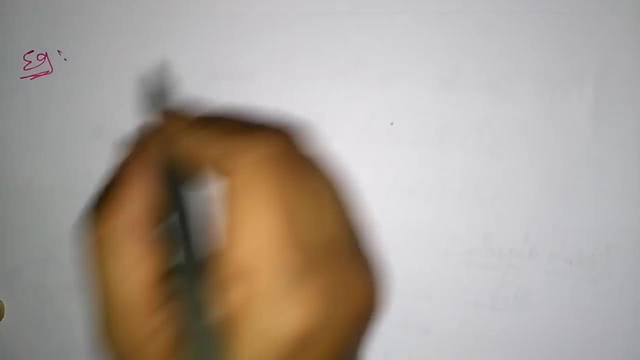 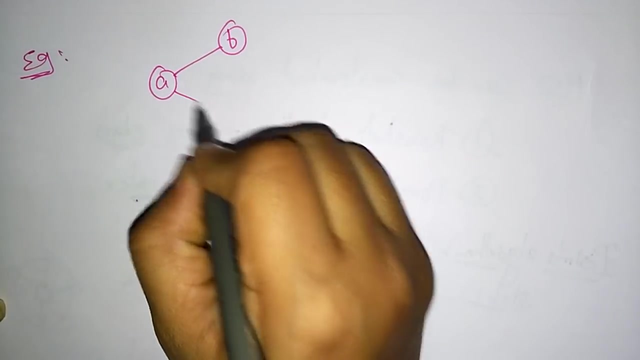 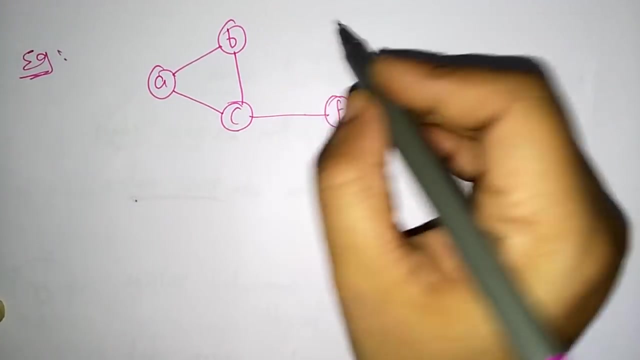 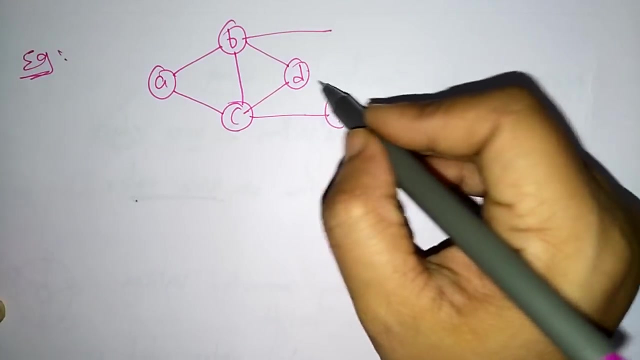 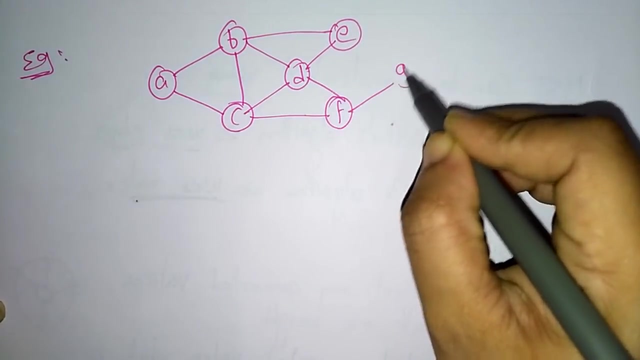 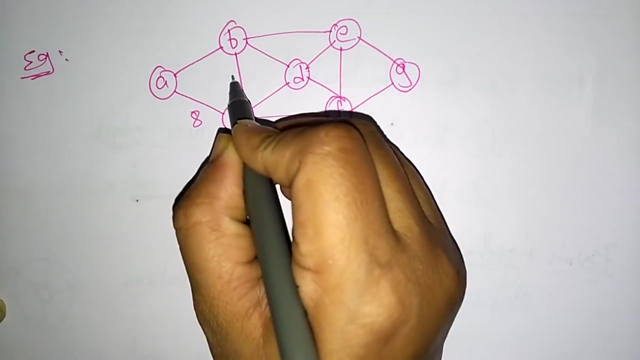 so this is one spanning tree. so i'm taking the graph, so now i have to connect, uh, convert this into minimum spanning tree. so graph is which is, with all closer loops, closed circuit. we can say, okay, so let's take and let me write the weights: eight, nine, four, and this is also eight. 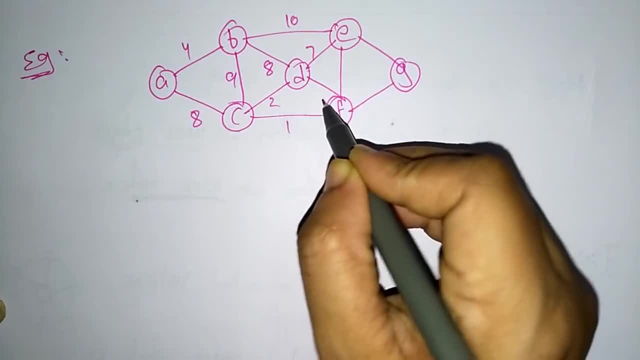 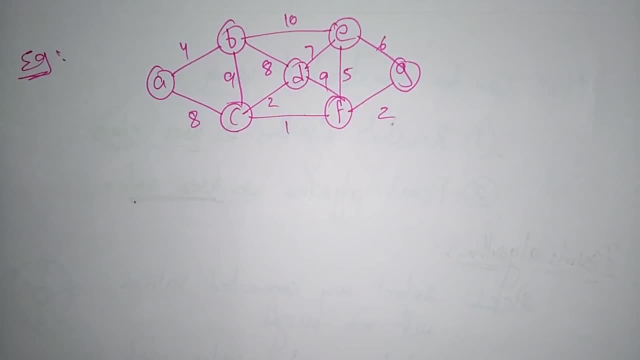 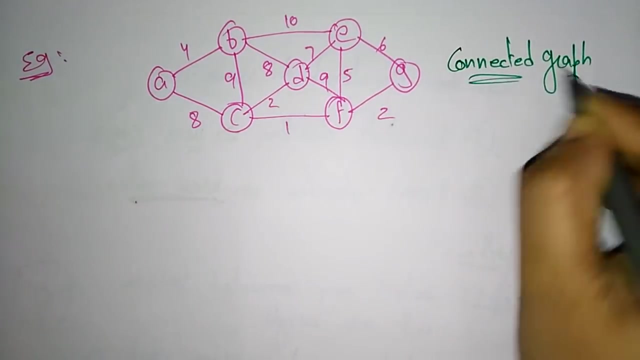 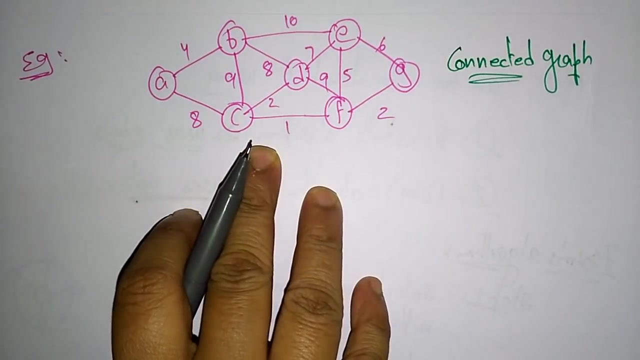 this is: let's take ten, seven, two, one. uh, let's take nine, five, six, two. okay, so this you call it as a connected graph. this is a connected graph, so one vertex is connected to another. what's it? so everything is in circuit. now let us write the step one. so now we are converting. 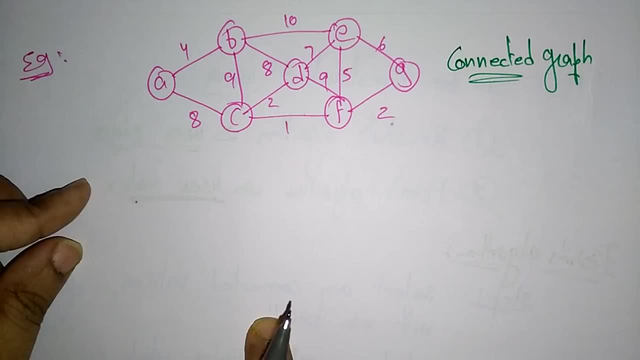 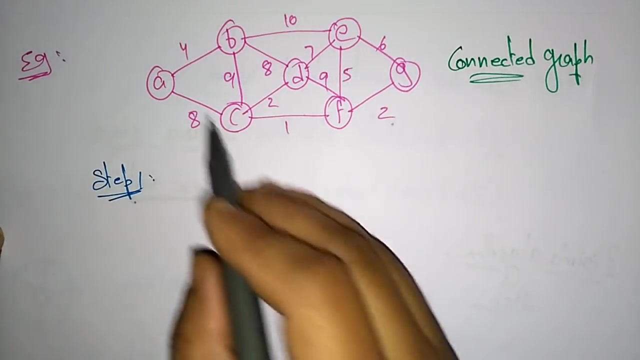 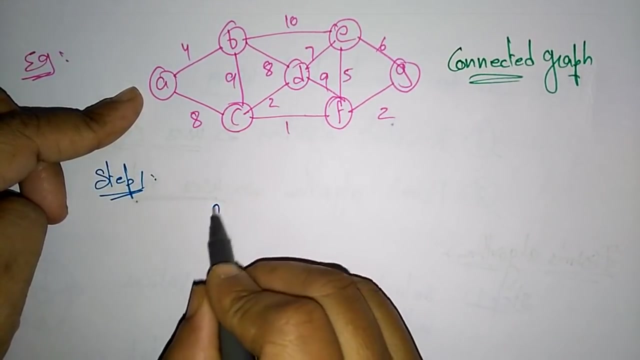 this graph into a minimum spanning tree by using prims algorithm, step one. so what is the prince algorithm? the step one? so we have to select any connected vertex with minimum weight. so let us take uh, suppose starting, we have, i'm taking a, so you have to take anything. so now i am taking the uh, a vertex. 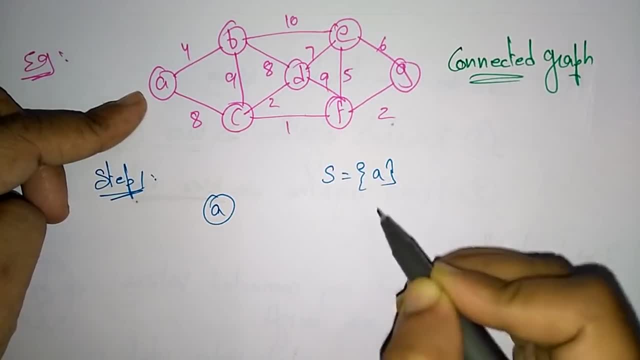 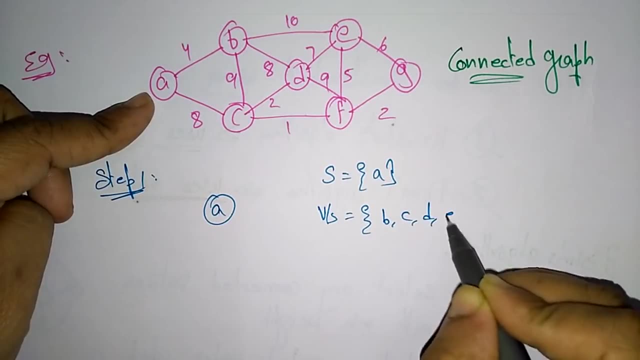 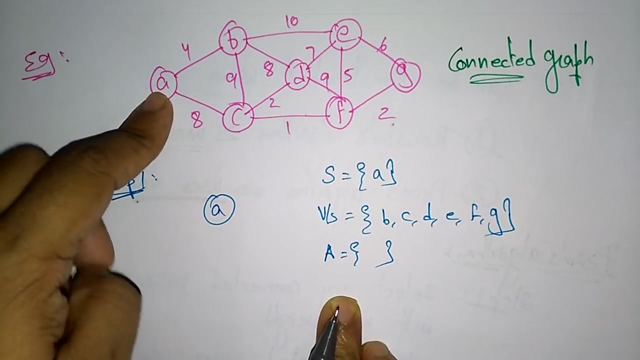 so here the set contains only one vertex a and the remaining vertices that are present in this graph, or b, c, d, e, f, g, okay, and the starting, the set contains an empty. so, uh, no, uh, connect connected. uh, vertices are there, not there. so let me write the lighted edge lightest. 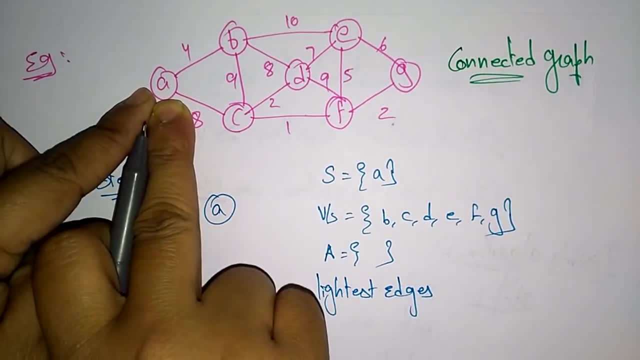 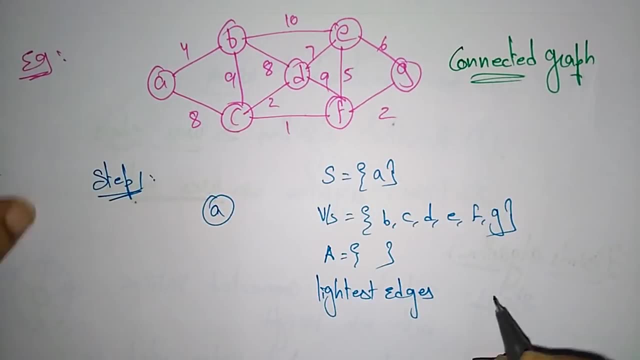 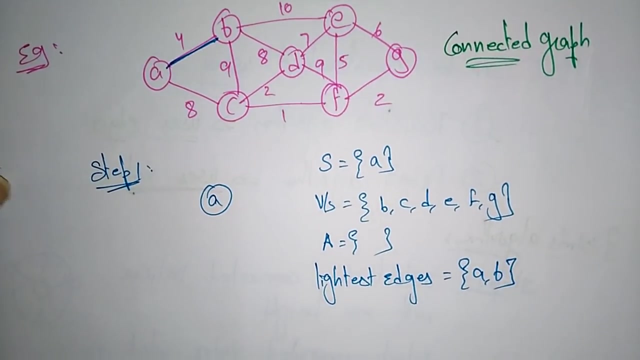 edge edges to this a. what is the lightest edges to this a? so either b, a or the lightest edges. this is the lightest edge, so that is a- b, so that i have to select in the step two. i am taking a b. okay, so now here the set contains: 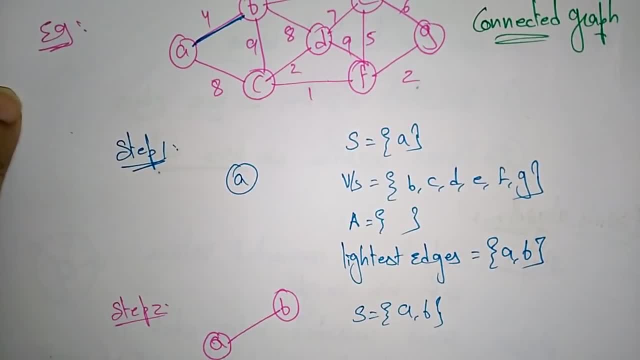 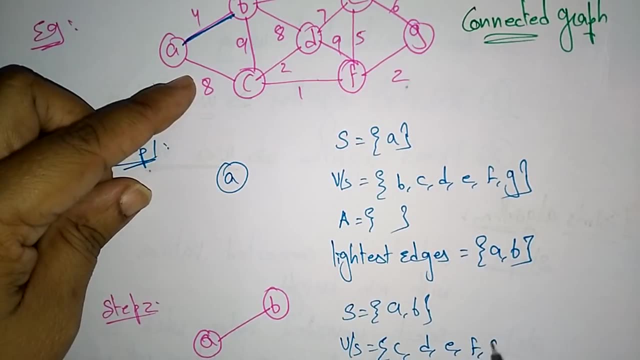 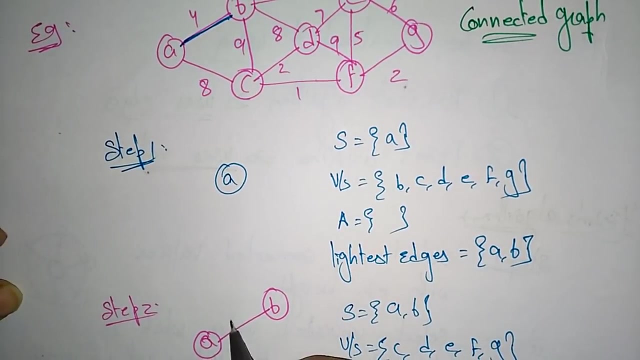 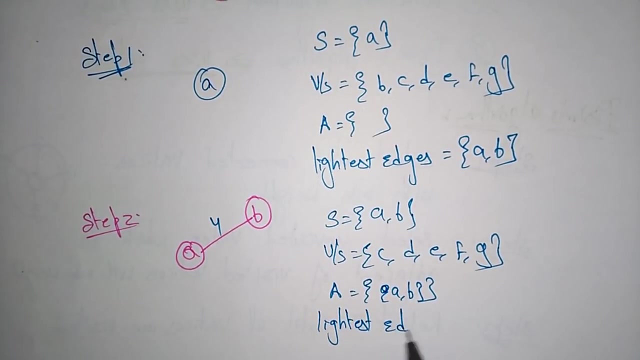 two vertices, a and b. set contains two vertices, a and b, and the remaining vertices are c, d, e, f, g. and what does the set contain? a comma b. so this is the weight four, and what is the lightest edges for this vertices? so the lightest edges are here, uh, 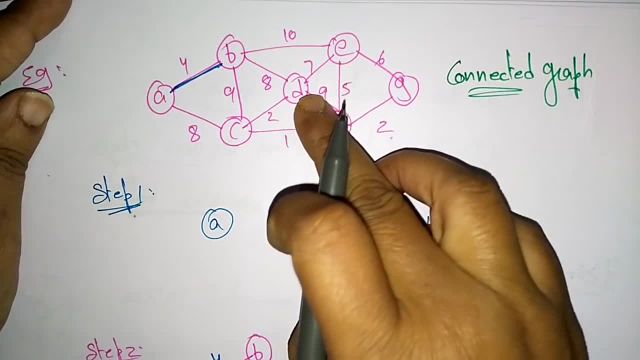 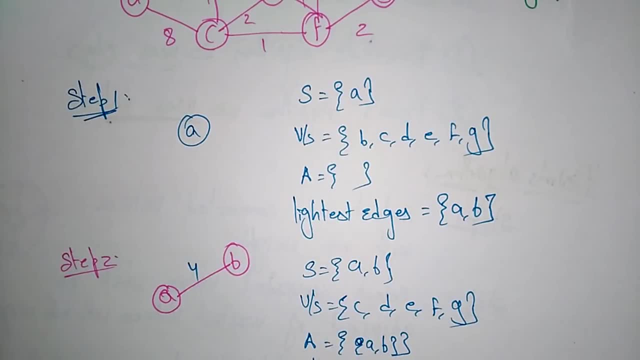 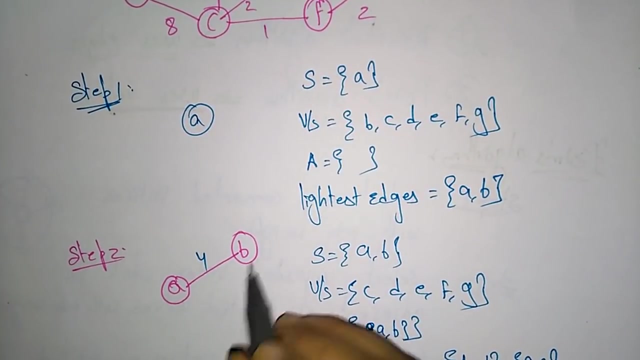 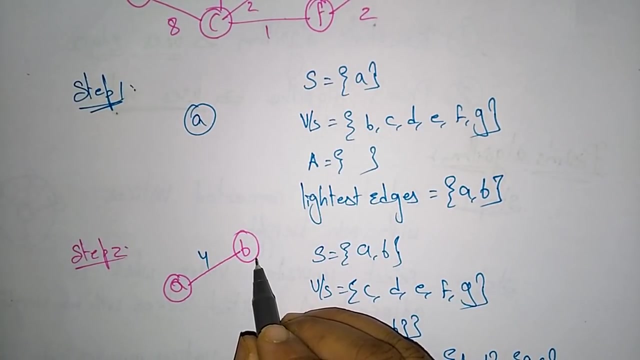 b, d or a, c, so both having the 8, BD or AC, BD or AC, so. but we have to connect from, we have to select. the Prim's algorithm means we have to select the unvisited vertex which is adjacent to the visited vertex with minimum weight. 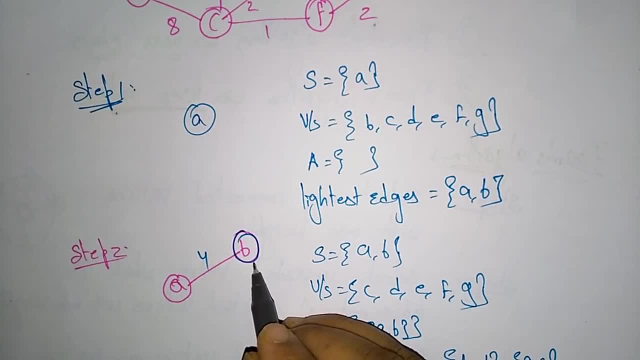 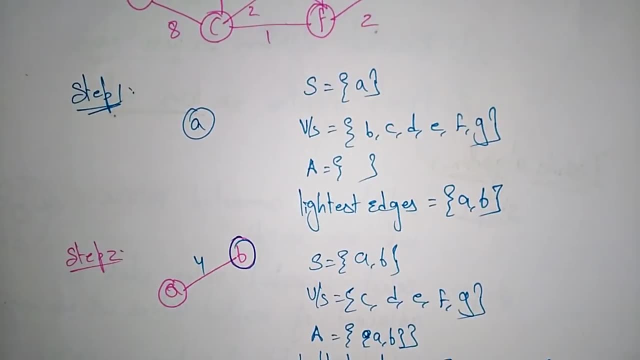 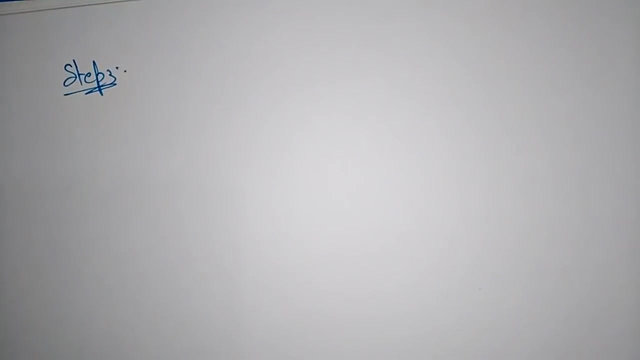 so we have to, from this we have to select which is adjacent to the visited vertices. so we have to select the vertices which is adjacent to B. so in the step 3, and step 3, so what is the step 3,? 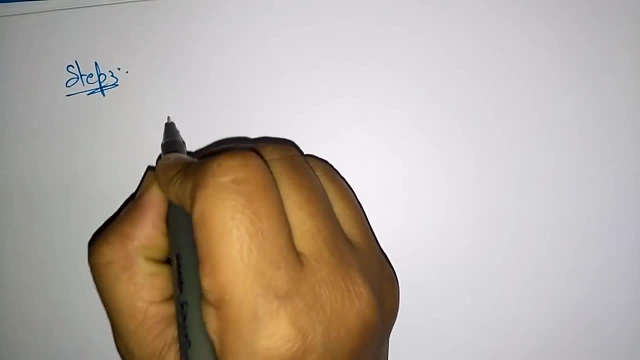 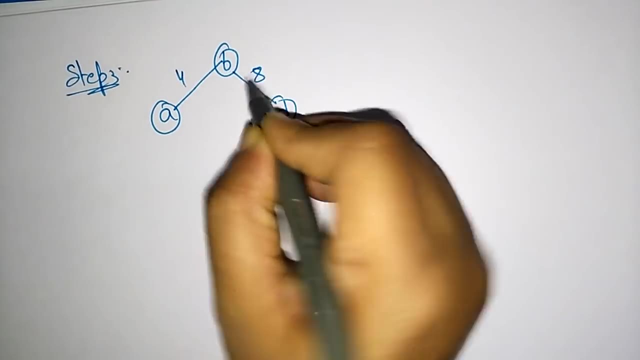 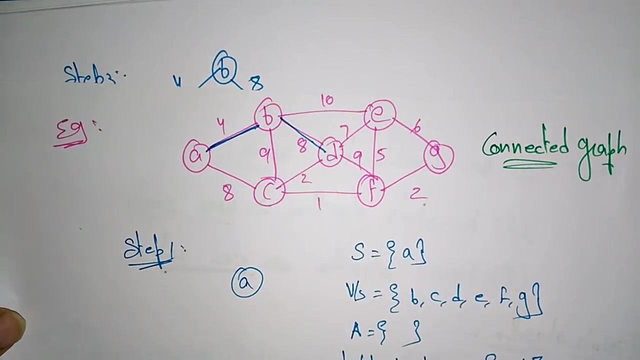 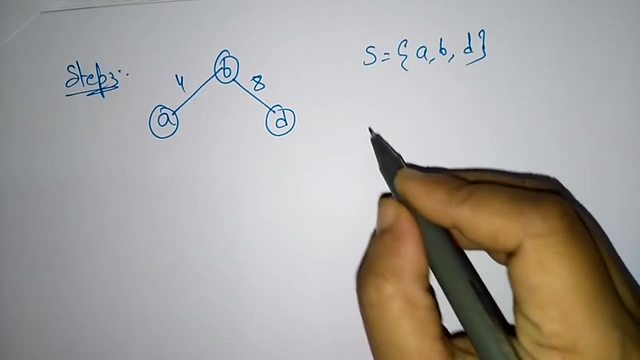 the step 3 contains, with 3 vertices, A, B, and this is D, 4,, 8,. okay, so we are reaching from A to D, so now, next, this set contains A, B, D, and the remaining vertices that are present in this graph are C, E, F, G. 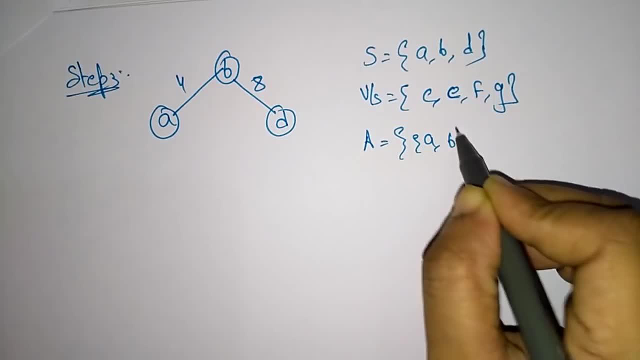 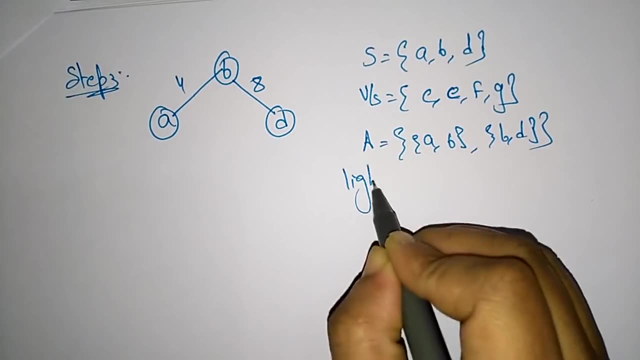 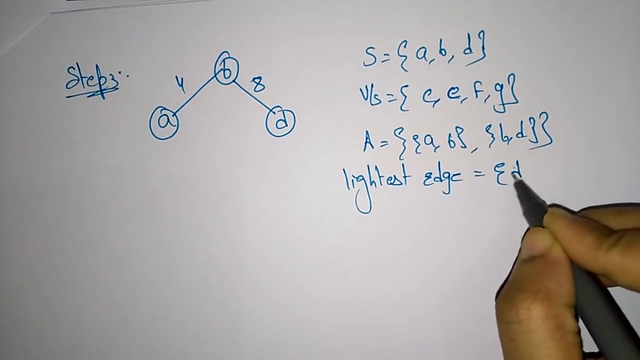 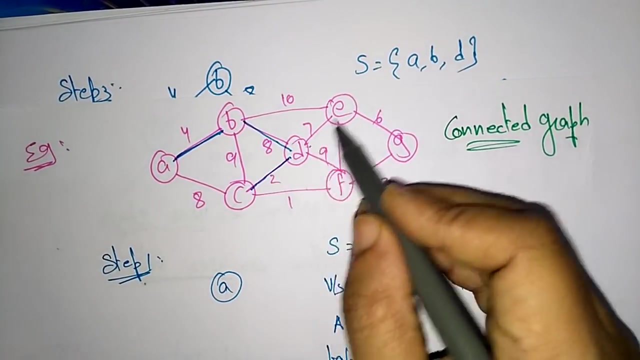 now the A set contains A, B- these are the two connected vertices- and then B, D. so next, what is the lightest edge to this? D lightest edge is D, C. why it is D, C, C. D C is 2, so whereas D is 7,, D, F is 9, so in this 3, the least weight is 2,. 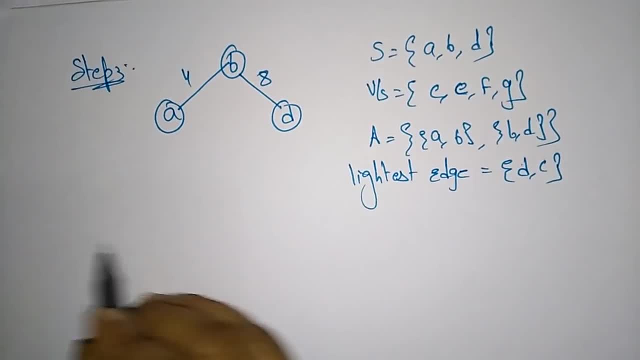 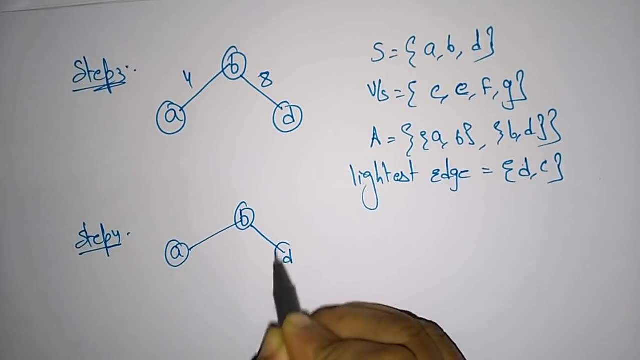 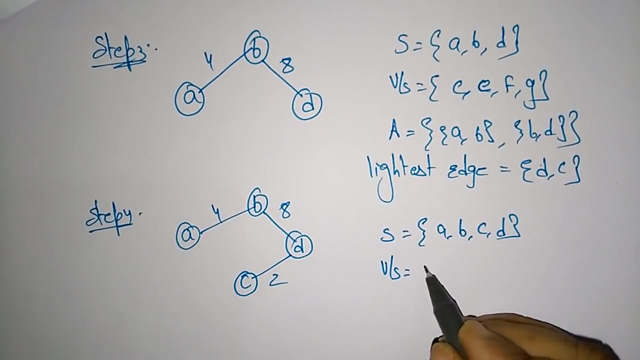 so we have to connect D, C. so step 4, A, B, D and this is C 4, 8, 2, now set contains A, B, C, D, 4 vertices, and the remaining vertices here are E, F, G. 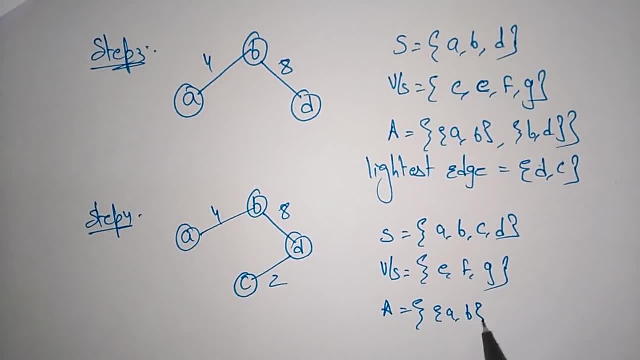 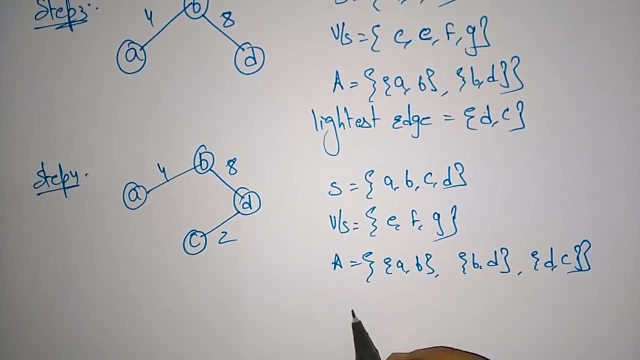 now the set is A, B, B, D and D, C. okay, what is the next lightest edge to C? so the next lightest edge to C, what is the next lightest edge to C, is C. 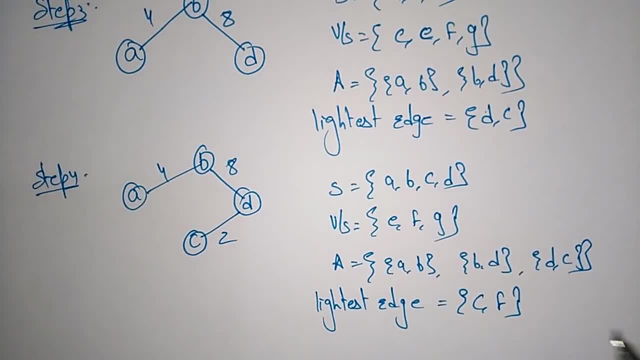 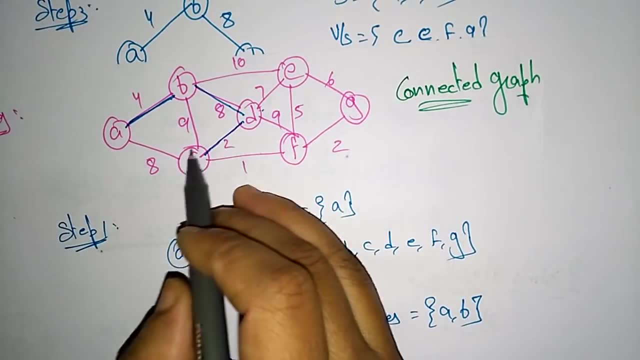 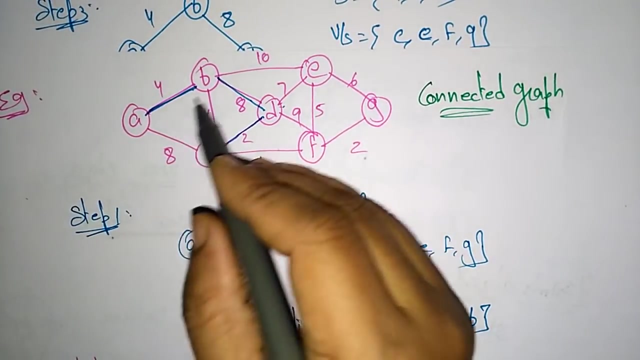 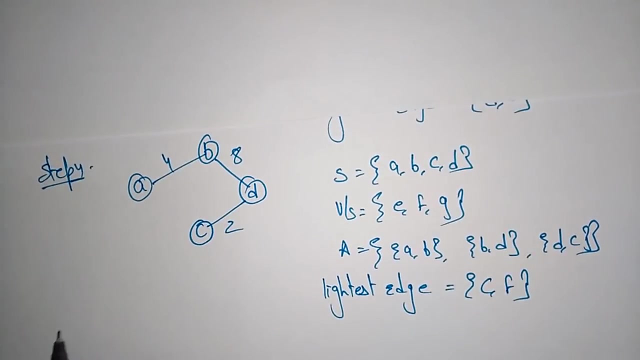 is c f, however, c f, just see here. so next option: c a. if we take c a, it comes to the closed loop, means it is a circuit, but the minimum spanning tree should not be allowed the circuit. so we have to select a, b, b, d, c, d, c and c f. so in step 5 let's write the graph: a, b, b, d, d, c and c f. 4, 8, 2. 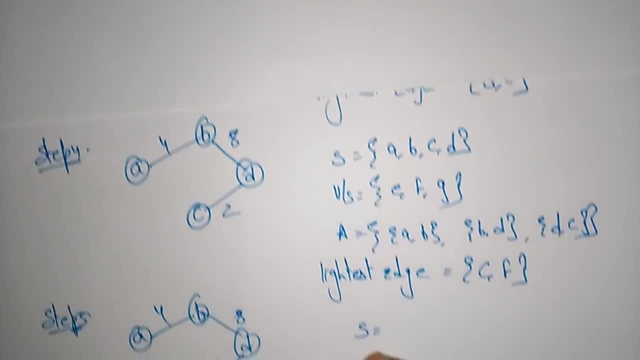 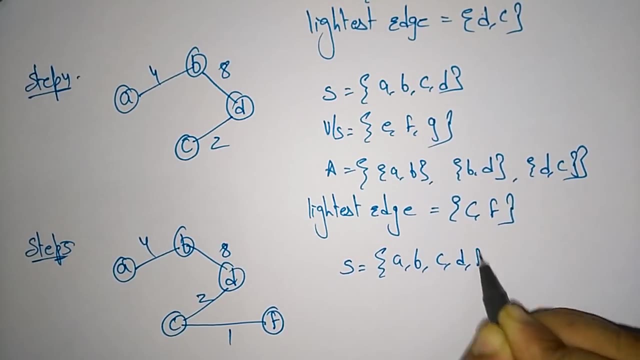 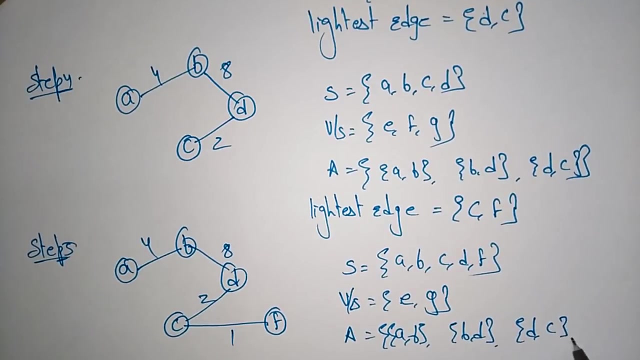 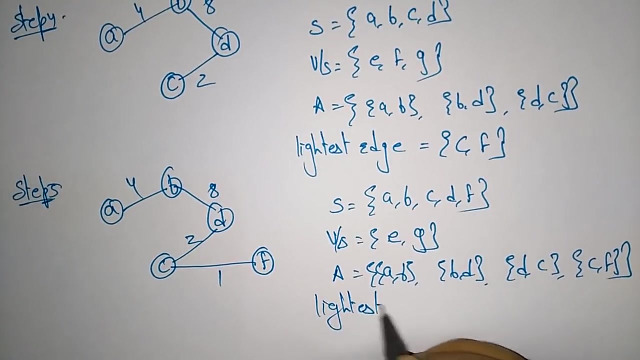 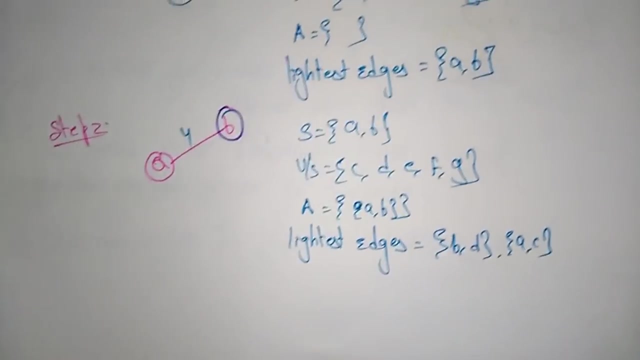 and this is 1. now this set contains a, b, c, d, f. what are the remaining vertices here? still, you are having e and g and the set contains a, b, b, d, d, c, c, f. next lightest edge is lightest edge, so next lightest edge is f, g. why it is f, g, c, f. 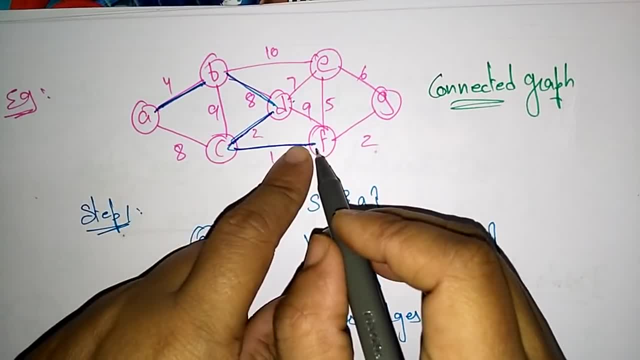 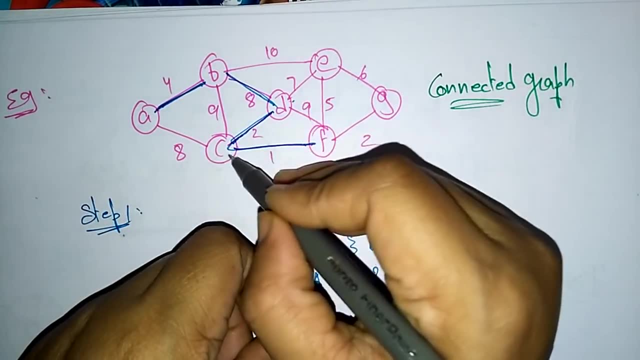 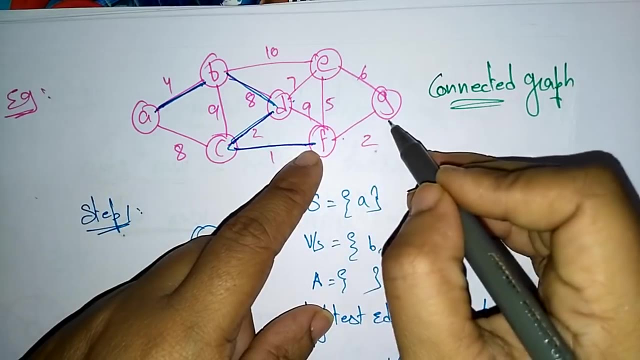 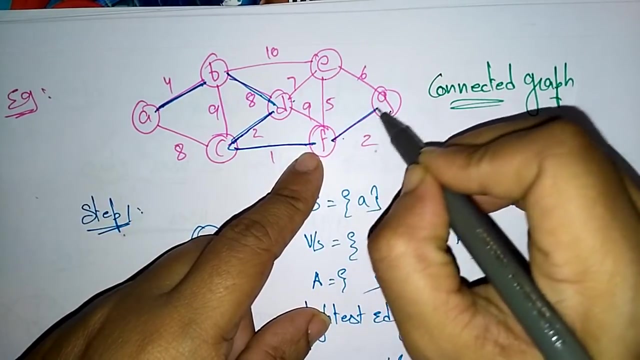 so in this, what is the adjacent to the f? we have to see the adjacent to the f are g, e and g. so if i take d, it becomes closed loop, closed circuit. so this is not possible. and if i take e, but when compared to e and g, which is the lightest weight, the less weight is the g, the two. so i am taking this f, g. 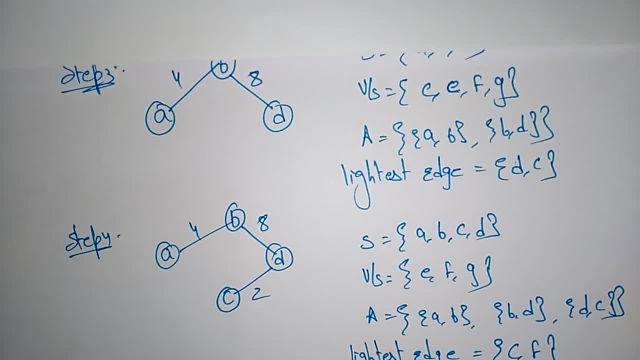 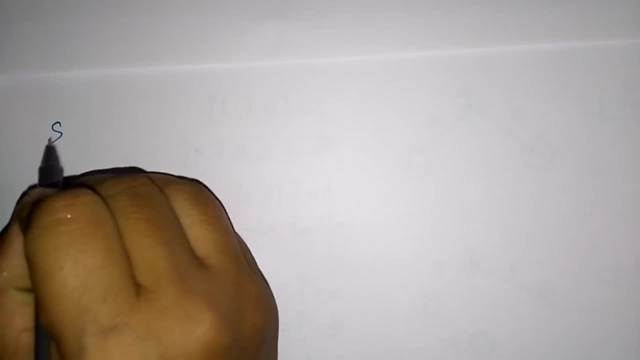 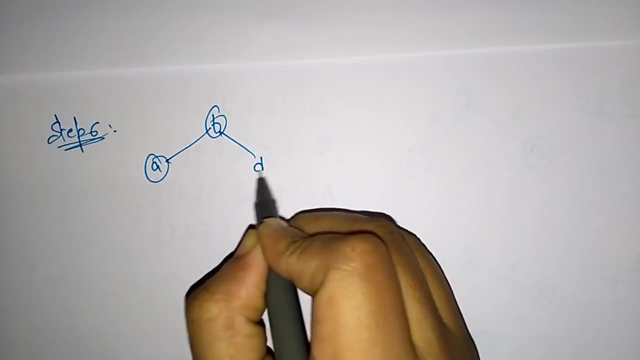 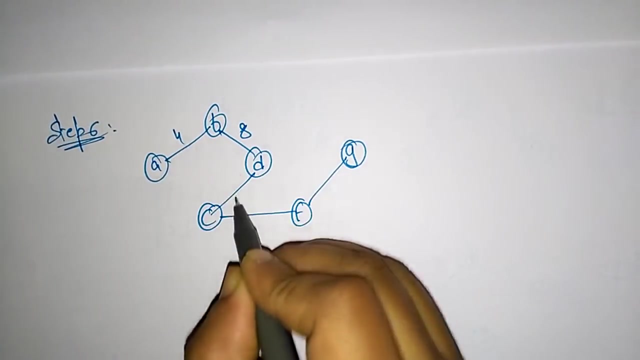 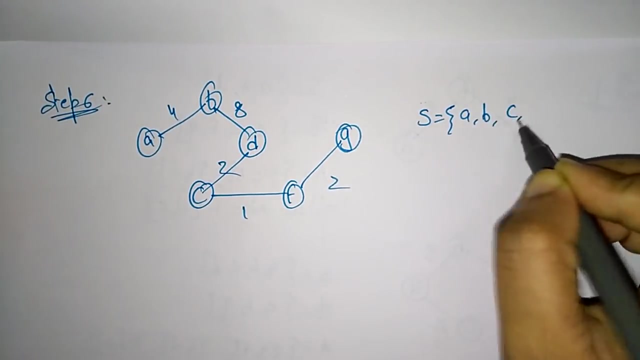 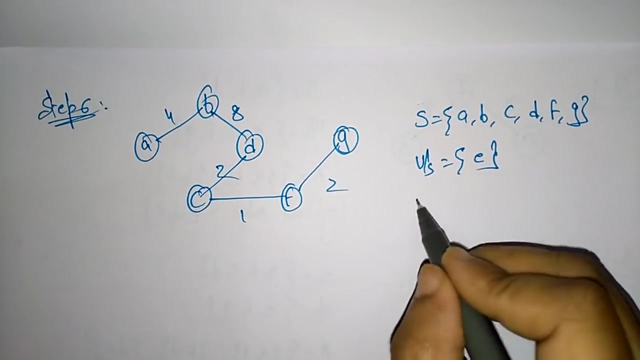 okay, so let me write that step six. so the step six is a, b, d, c, f, g. so this is four, eight, two, one, two. now coming to the sets. so s contains g, g, a, b, c, d, f, g. what is the remaining vertices? only e is remaining. and what is the complete sets? you? 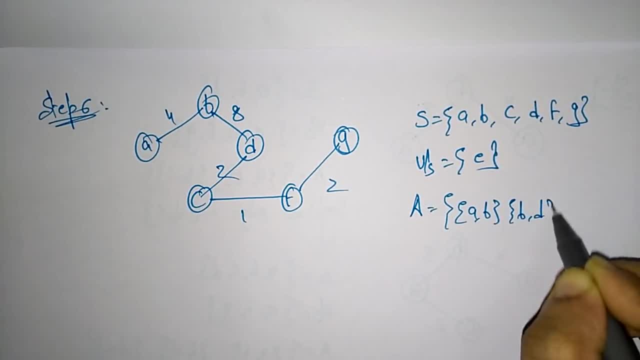 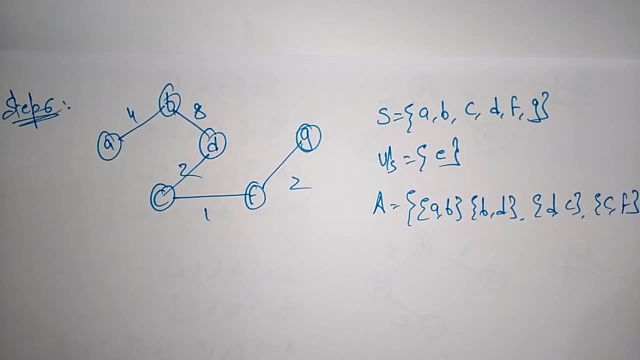 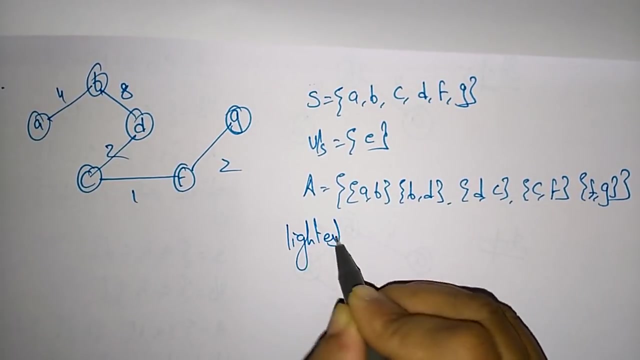 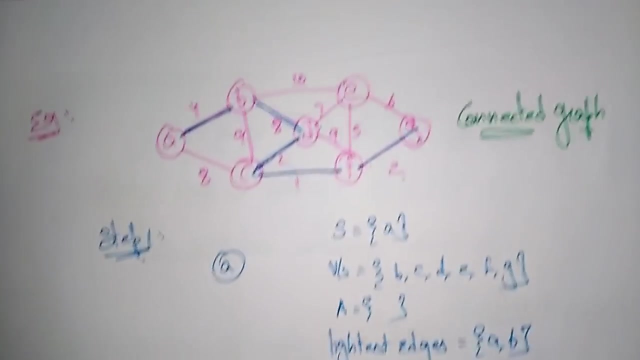 are having a, b, b, d, d, c, c, f and f, g. okay, now what is the lightest edge for the g? so we have to select from g. so the lightest edge is f, e. so, when compared to here, uh, f, g and uh e, this is the.